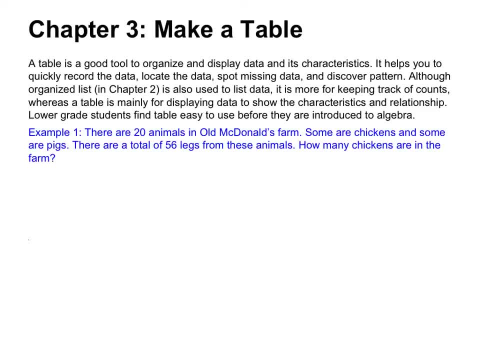 There are 20 animals in Old MacDonald's farm. Some are chickens and some are pigs. There are a total of 56 legs from these animals. How many chickens are in the farm For more grown-up students who have learned algebra? they can quickly solve this problem. 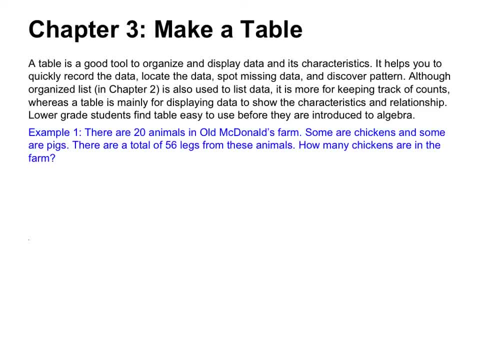 But what if you have not learned algebra? Perhaps a table will come in very handy. This is a table that we're going to use. In this table I have listed a row for the count of chickens, a row for pigs and a row for chickens. 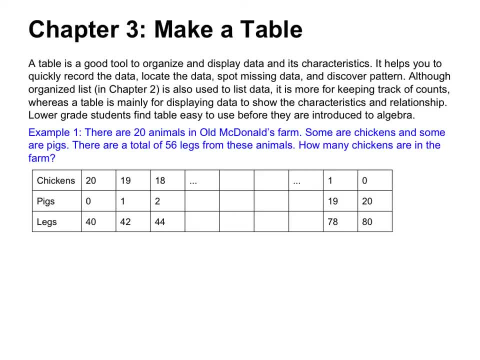 In this table I have listed a row for the count of chickens, a row for pigs and a row for pigs. In this table I have listed a row for the count of chickens, a row for pigs And a row that records how many legs are out there. 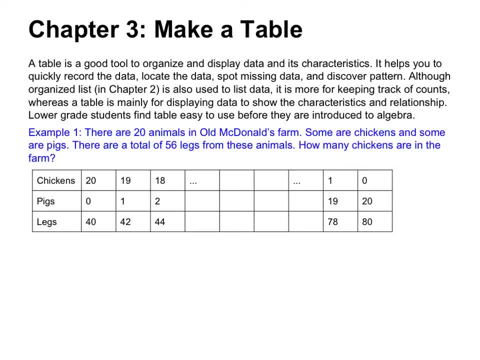 And this table will show me the trend. So I can pretend that there are 20 chickens and there are no pigs, because I have a total of 20 animals. So if I have 20 chickens, then I will have no pig at all. 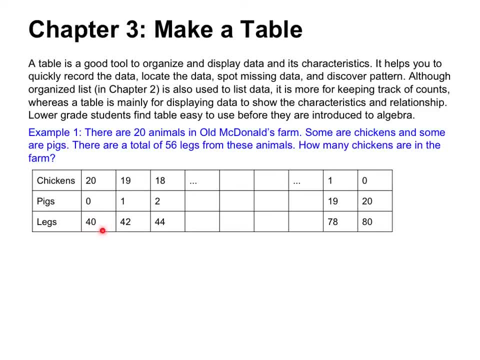 And then I count how many legs are out there. So all the legs must be from chickens. Each chicken has two legs, so 20 chickens will have 40 legs. And then what about only 19 chickens and 1 pig? Now, if I have 19 chickens and 1 pig, then I can record 42 legs out there. 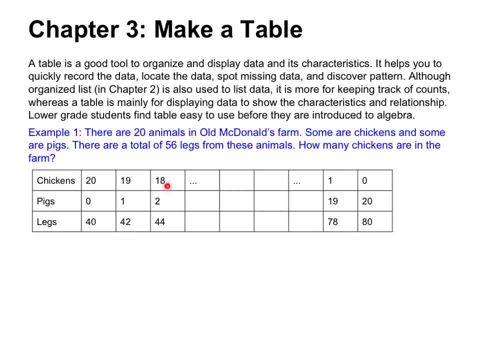 Or maybe there are only 18 chickens, 2 pigs. then there will be a total of 44 legs. Now you don't have to list all the possible combinations of chickens and pigs. Now you don't have to list all the possible combinations of chickens and pigs. 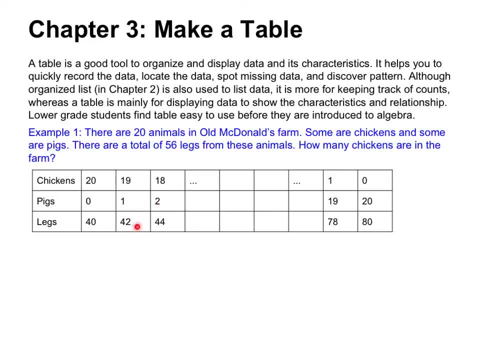 But just list some of the numbers out and then see the trend, see the pattern. I also listed in the far end here, in the other extreme, that I will have no chicken and all 20 animals are pigs And in that situation I would have 80 legs, because each pig has 4 legs right. 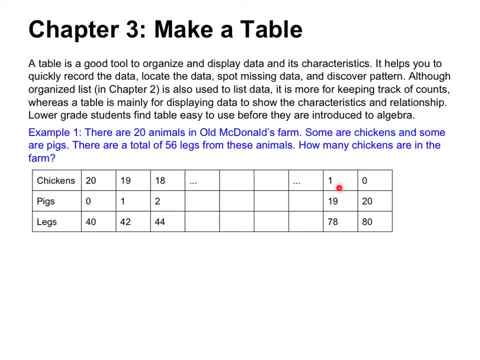 And I can also increase the chicken count by 1.. Then I would have lose 1 pig just to trade for the chicken And I would have counted 78 legs. Now I want you to pay attention to the number of legs As we move from more chickens to less chickens, from less pigs to more pigs. 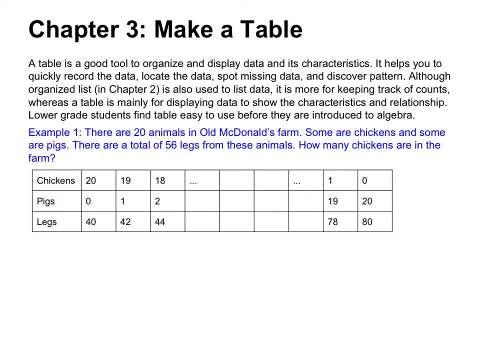 what happens to the number of legs? Do you see that every time when we lose 1 chicken and gain 1 pig, we gain 2 legs here? Or, on the contrary, every time when we gain 1 pig, we gain 2 legs here? 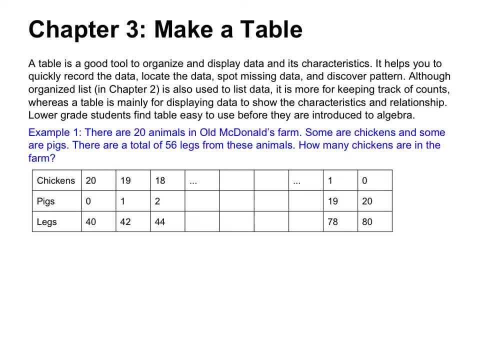 On the contrary, every time when we gain 1 chicken and lose 1 pig, we lose 2 legs. Why is that? You probably can answer it: Because a chicken has only 2 legs and a pig has 4 legs. So if you trade a chicken for a pig, then you have gained 2 legs. 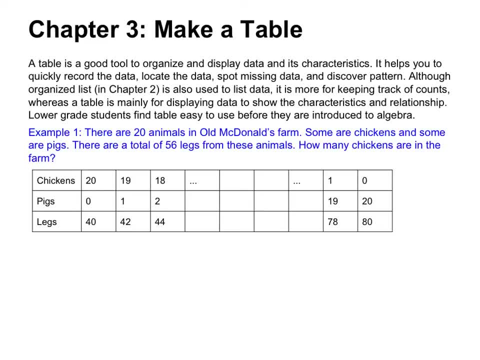 Okay, use this table. Now let's focus on our problem. We want to have 56 legs. Now, none of these is 56. But from this table you can see that one extreme is 40 legs, The other extreme is 80 legs. 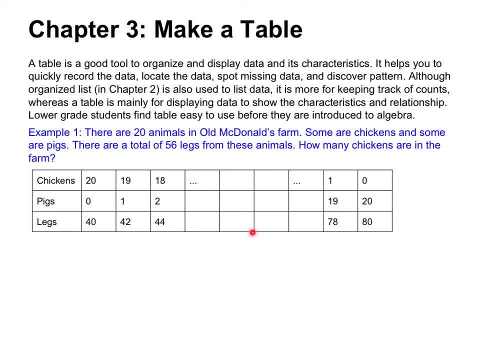 So somewhere in the middle is 60 legs. That's in the middle, But 56 is a little bit less than 60. So in the situation of 60, then I would have. So let's write down 60 legs, If I have 60 legs. 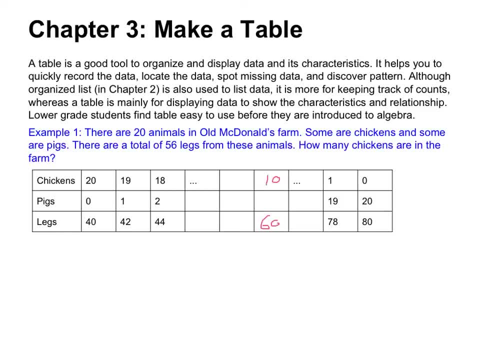 then I would have half chicken and half pigs, like 10 and 10.. But remember that every time when I gain a chicken and lose a pig, I lose 2 legs And I'm looking for 56. That means, from 60, I need to lose 4 legs. 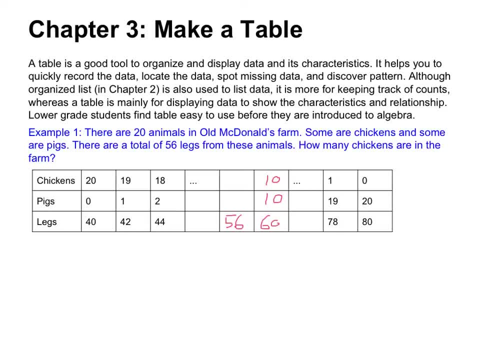 That means I need to have 2 fewer pigs and 2 more chicken. From what I got so far, that would do 56. And then you can do a quick multiplication to do 12 times 2,, 8 times 4,. 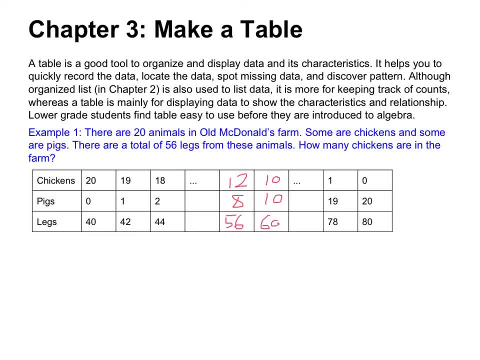 add them up to see if you really get 56. And you should. So there are 12 chickens. So in this example we see that we can use a table to list the numbers and then see the trend, see how numbers are related to one another. 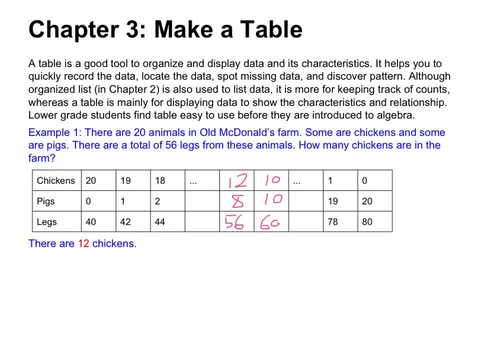 And then use somewhat estimation to help us to locate the answer and to fill in the table to get the final answer. All right, Here's one example for you to try out: 32 coins made up of quarters and dime has a total value of $6.20. 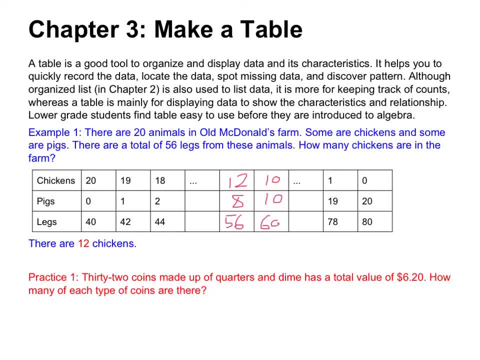 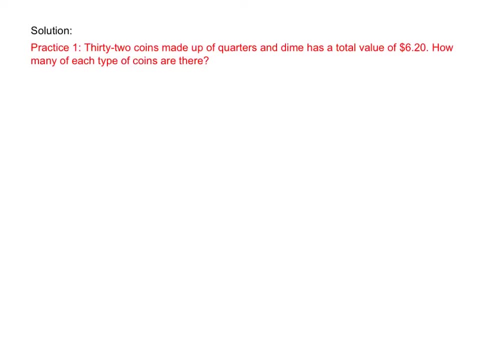 How many of each type of coins are there Now? each quarter is $0.25 and each dime is $0.10.. So how many of each? Pause the video and try it out When you're ready, move on. So here's the solution for the previous practice. 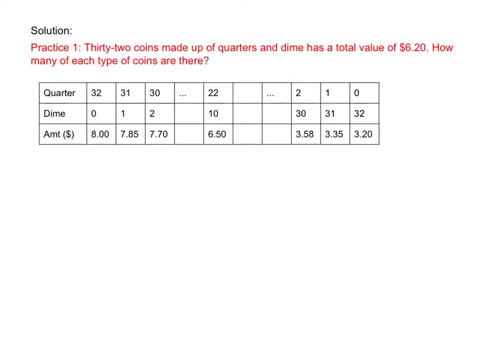 I use a table to list all the possible ways I can have the coins. So in one end I can have all quarters and no dime, and then I would lose one quarter and gain one dime each time, and then going from left to right And at the end 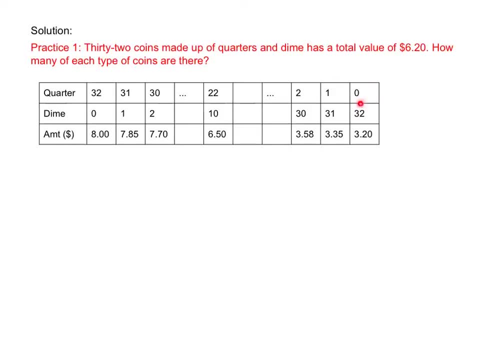 my combination is: I have 0 quarter and all dimes And in each case I recorded how much the dollar amount is. And after writing a couple of columns like this and here on the other end, I pretty much see the trend. I know that for each quarter that I lose, to gain one dime. 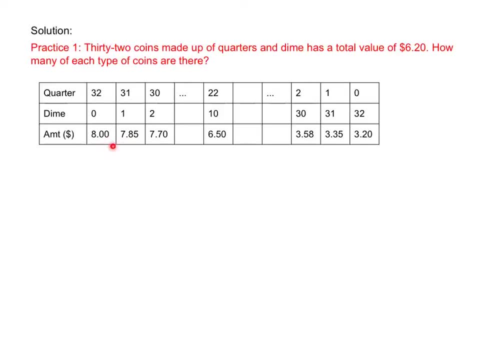 I lose a net of $0.15.. And that makes sense, because a quarter is $0.25 and a dime is $0.10.. So if I lose $0.25 and gain $0.10,, my net loss is $0.15. 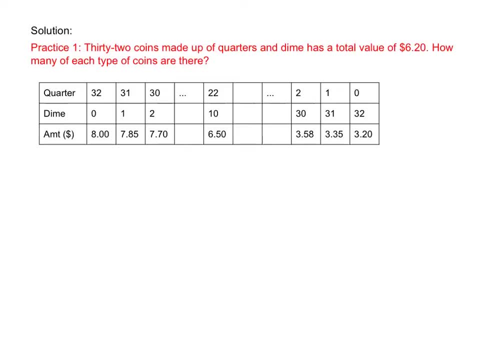 Now the number that I need is $6.20.. $6.20 is between $8 and $3.20, but it's closer to $8 and a little bit farther from $3.20.. So instead of trying a middle number like 16 of each coin, 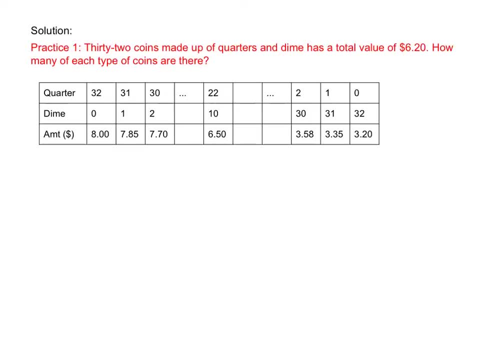 I try a number that is closer to the left. So I pick 20, 2 quarters and 10 dimes and see what these two will add up to, And I found out that these two will add up to $6.50. 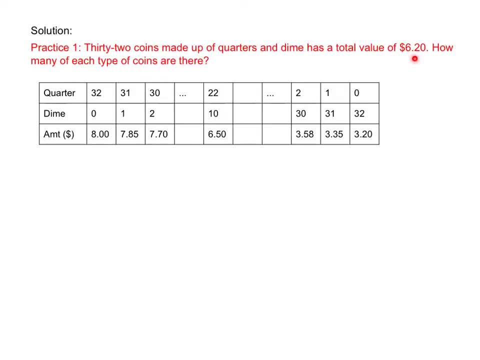 I'm still away from $6.20, but I know I'm quite close to it And all I need to do is to switch some coins so that the net change is $0.30, because now I have $6.50.. I want to lose $0.30 to get to $6.20.. 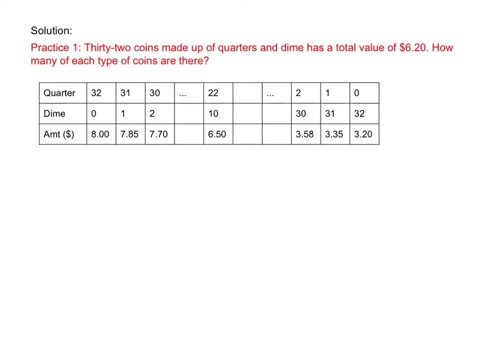 So this is what I can do, Since I need $6.20, I need to lose 2 quarters, so I would have 20 quarters, and then I would gain 2 dimes, so I would have 12 dimes. Then I should get $6.20. 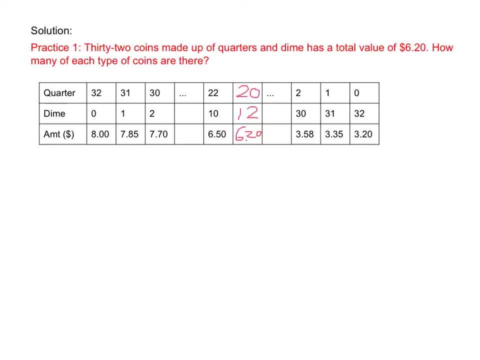 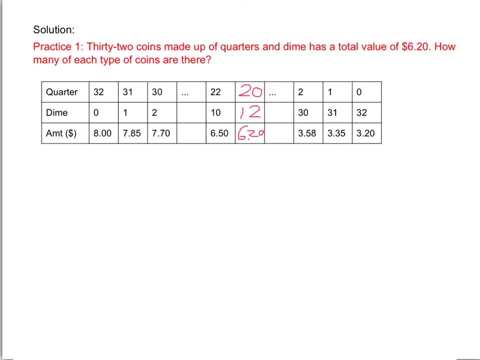 And I can quickly add up the value: 20 quarters means $5.. 12 dimes means $1.20.. Yes, and they add up to $6.20.. And I'm done. So the answer is 20 quarters and 8 dimes. 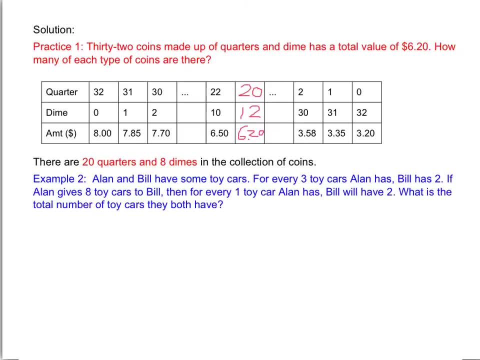 in my collection of coins. Okay, so here's another example of using table. Alan and Bill have some toy cars. For every 3 toy cars Alan has, Bill has 2.. If Alan gives 8 toy cars to Bill, then for every 1 toy car Alan has. 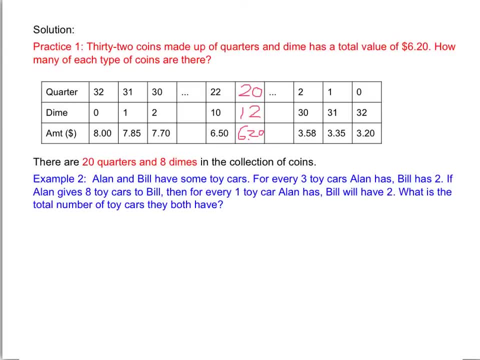 Bill will have 2. What is the total number of toy cars they both have? Well, you can pause the video and try to read this problem again to get yourself familiar with the situation. Okay, we use the table to record the possible ways that they can have. 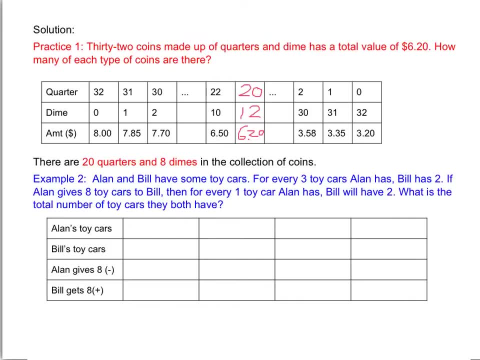 3 toy cars. For every 3 toy cars Alan has, Bill has 2.. So that makes us think about maybe Alan has 3,, Bill has 2,, or Alan has 6,, Bill has 4,, or as long as the ratio is 3 to 2.. 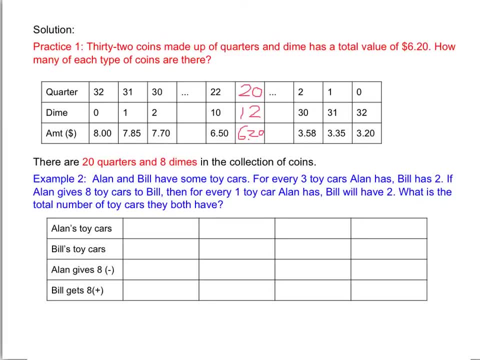 However, it's impossible for Alan to have only 3 toy cars, because if he gives 8 toy cars to Bill, that means he needs to have more than 8 toy cars, 8 or more. So we cannot just try like 3 toy cars, 6 toy cars. 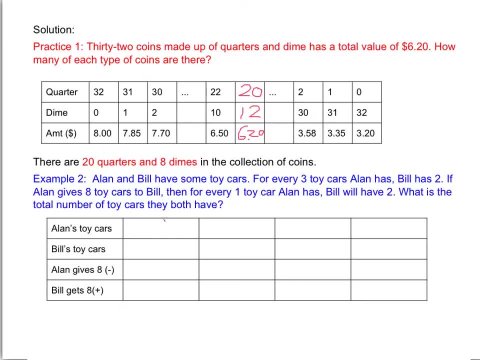 So the minimum number of toy cars that we want to try out is 9.. Again, the ratio is 3 to 2.. So if Alan has 9 toy cars, then Bill will have 6 toy cars, Or if Alan has 12,. 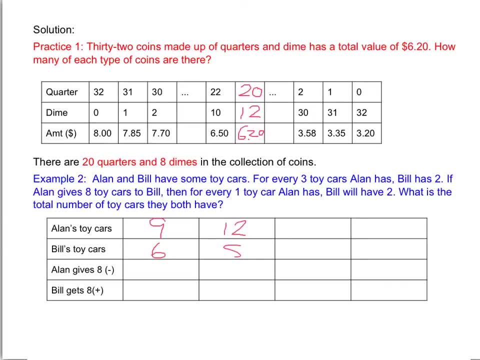 then Bill will have 8,, 15, and 10,, 18, and 12.. All these combinations show a ratio of 3 to 2.. Now which one is the right answer? Sometimes we will need to keep trying until we get it. 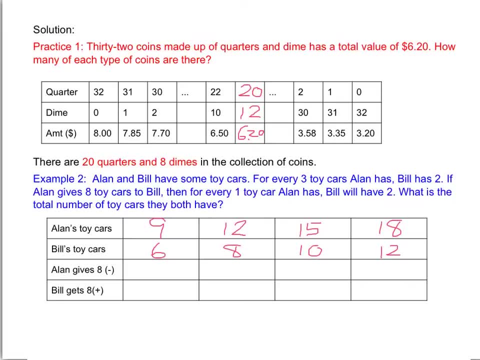 Sometimes when we see the pattern we can jump a little bit farther to get ourselves land on the answer faster. So let's examine the situations that if Alan is to give 8 toy cars out, so we need to subtract 8 from Alan's collection. 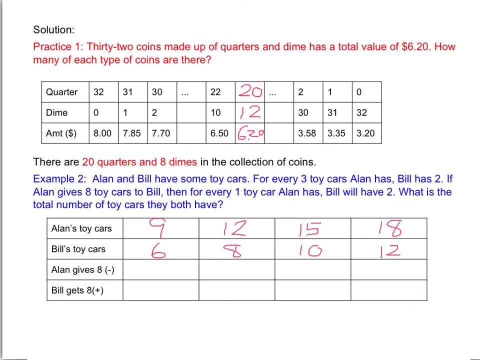 then Alan would have only have 1 toy car left, because he gives 8 out And Bill Bill gains 8, so add to 6, then Bill will end up with 14.. Then let's examine the condition It says after Alan gives 8 toy cars to Bill. 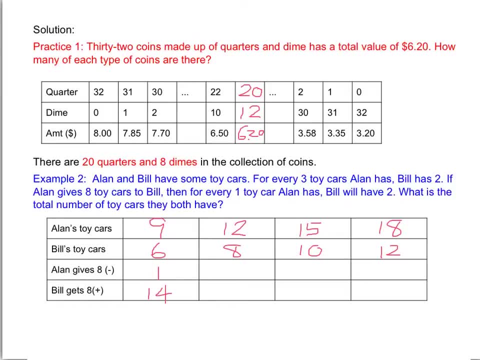 then for every 1 toy car Alan has, Bill will have 2.. Now, for every 1 Alan has- in this case, Bill does not have 2. Actually, Bill has more than 2. So this is not the case that we want to look for. 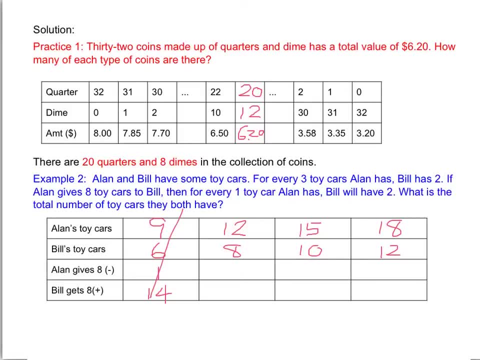 Then let's move on to the next one, After Alan gives 8 out. so subtract 8 from 12, then he will have 4 left. And Bill started with 8, gained 8, then Bill has 16.. Again, this is not 1 to 2 ratio. 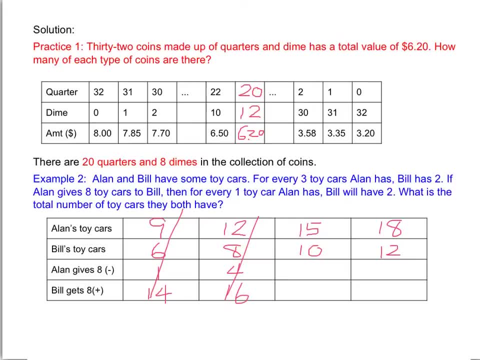 Alright, So we'll cross this off again and keep trying the next one in the same fashion. And 15 subtract 8 is 7,, 10 gain 8 is 18.. Again, not 1 to 2 ratio. Look at this one. 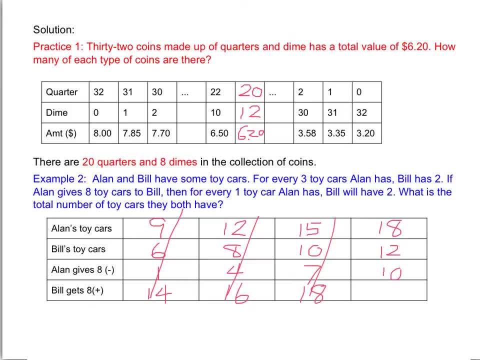 18 subtract 8 is 10, then 12 plus 8 is 20.. Now 10 to 20 is the ratio of 1 to 2.. Finally we found it. So this is the answer. So initially Alan has 18,. 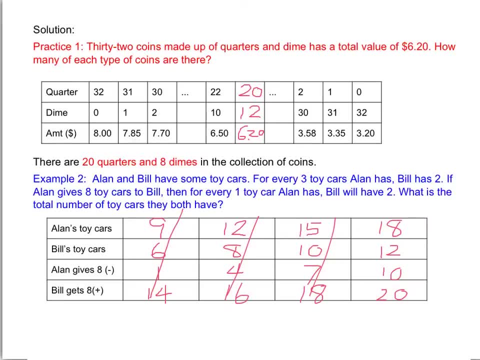 Bill has 12.. After giving to Bill now, Alan has 10 and Bill has 20.. But in either case, since we are asked to find the total number of toy cards they both have, you can use the initial case or use the afterward one. 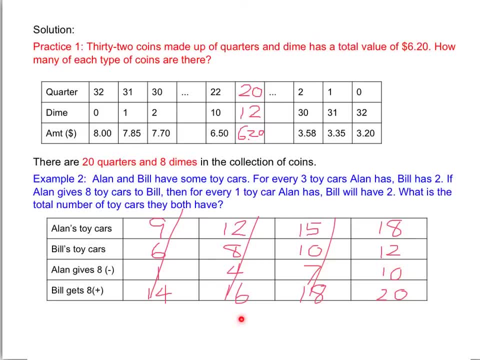 They both will evaluate to a total number of 30 toy cards. Now notice that in this problem we use tables to try different combinations. Sometimes we may not just get it right away. We have to keep trying several times Because I know that I will get the answer here. 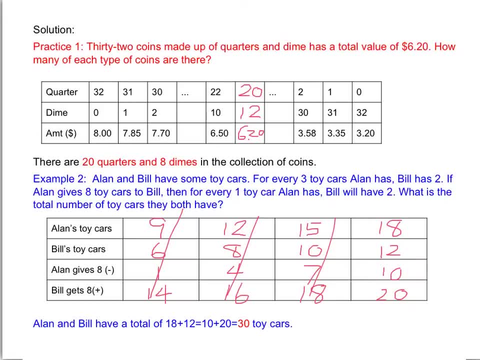 that's why I only have 4 columns, But sometimes you may need to keep extending your table until you get the answer. But you can also look at the trend like from here to here. You see the ratio. The first one is 1 to 14,. 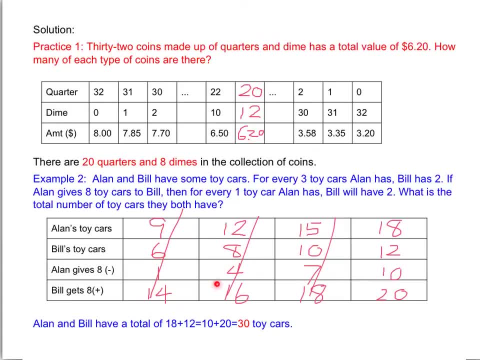 which is a very, very small ratio. Then we have 4 to 16. This is close to 1 fourth, Then 7 to 18.. Now this is a little bit more than 1 third. So you see how we change the ratio over. 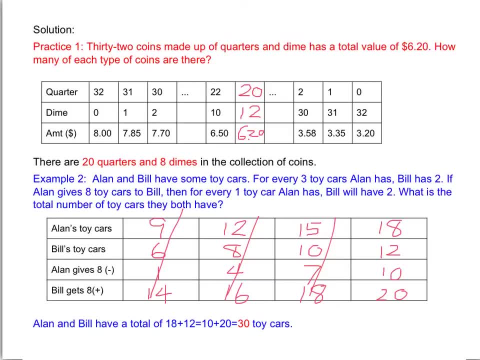 when we change the numbers in the beginning case, So we know that we are going in the right direction. Sometimes, if you see the number is so full, so far away from what you are looking for, you can jump a couple of columns and just try some other numbers. 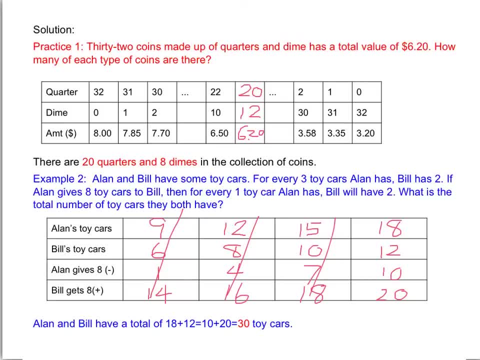 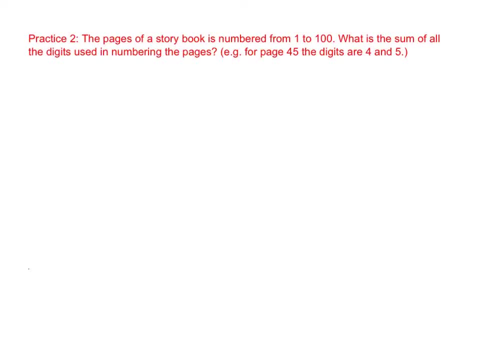 to get you to land on the answer faster. Okay, here is another practice for you: to try: Pause the video and when you are done you can resume it. So here is the solution for practice 2.. The pages of a storybook is numbered. 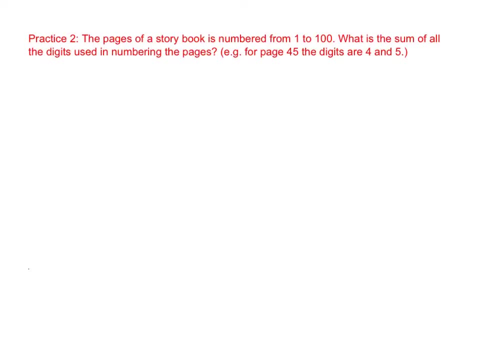 from 1 to 100.. What is the sum of all the digits used in numbering the pages? For example, for page 45, the digits are 4 and 5.. So you are adding the digits of all the page numbers. So page 1 is 1,. 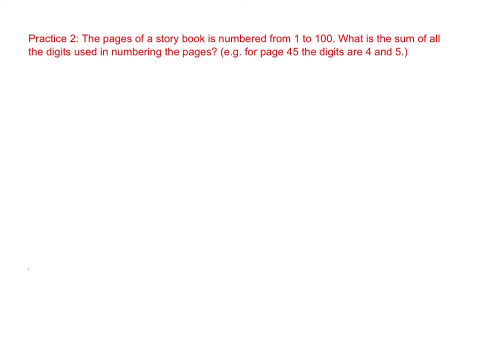 page 2 is 2,, page 10 is 1 and 0,, page 45 is 4 and 5, and so on. So you are adding all the digits up. So what is the sum of all the digits? Well, at first glance. 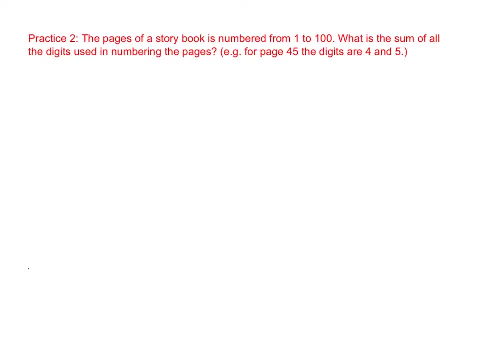 it sounds so complicated, But perhaps we can use a table to help us keep things organized and see the pattern. That's the most important thing: to see the pattern. Okay, so in my table I have two columns, I have page numbers. 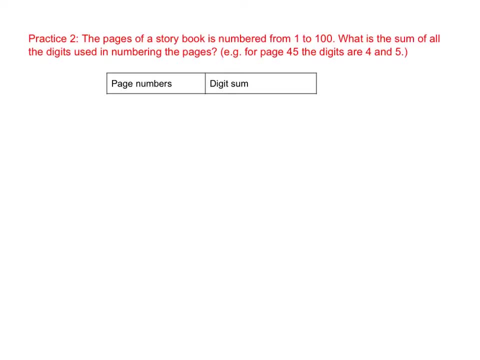 and the digit sum. So let's look at the page numbers grouped by another group. The first group that I look at is the first 10 pages, Pages 0 to 9.. And I can find out the digit sum is 45.. 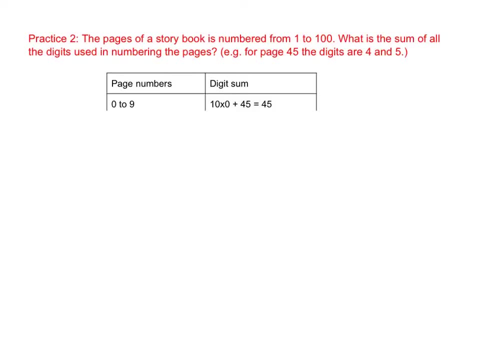 You add up 0 to 9, you get 45. I'll explain my expression in a second. It looks kind of weird, but I'm looking at a pattern right now. So in my second group of the pages, I am looking at pages 10 to 19.. 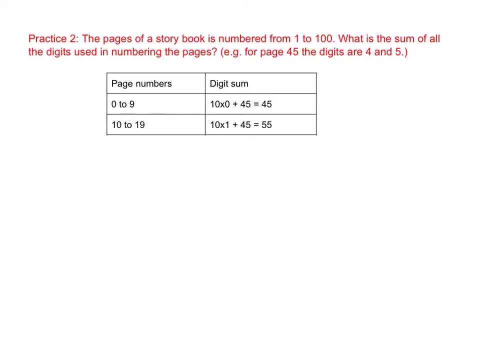 And if I add up all the digits from 10 to 19,, I see something interesting, Because all these digits, all these numbers, begin with 1, so I have an extra 1 as my digit in each page, So I need to add 10 ones. 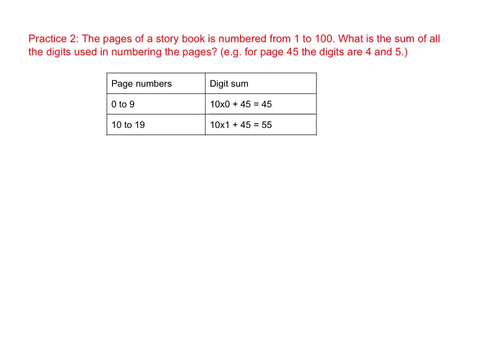 because of the 10, 11, because of the 10th place is a 1, so I need to add 10 ones on top of my 0 to 9, which is 45. So I have a total of 55. 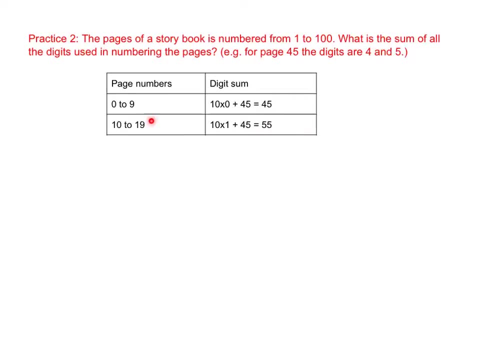 as the digit sum In this group of pages. And then I continue to move on. Now I consider pages 20 to 29.. Again, from page 0 to 9, like the digits 0 to 9, I always get 45.. 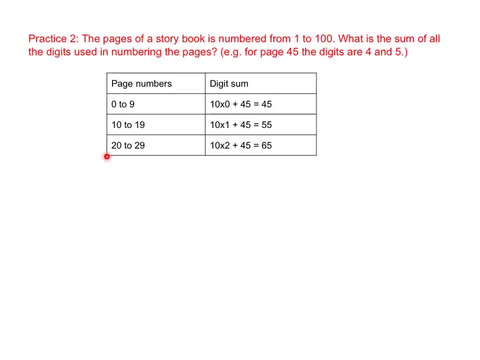 But now, for each page I have an extra 2. And there are 10 such pages. So I'm going to do 10 times 2 and add to 45 and I get 65. And I can keep doing several times. 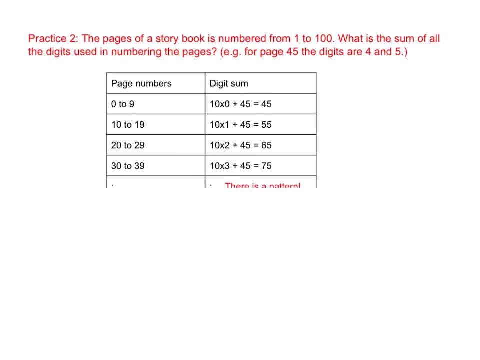 Until I see a pattern. Do you see a pattern here? Yes, The pattern is in my expression. to come up with the sum, I always have 45 at the end, because my 1's place is always 0 to 9.. That's in my 1's place. 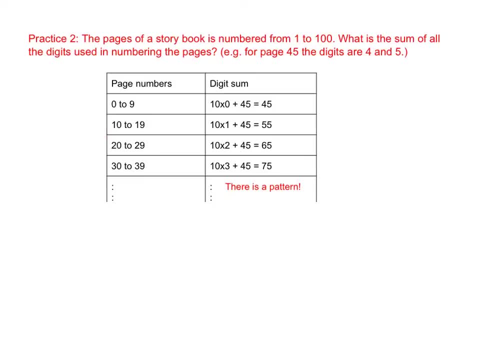 But my 10's place, depending on which group I'm looking at. I begin with the group that has no 10's place, So I have 10 times 0. Then I move on to the 10's place that is 1.. 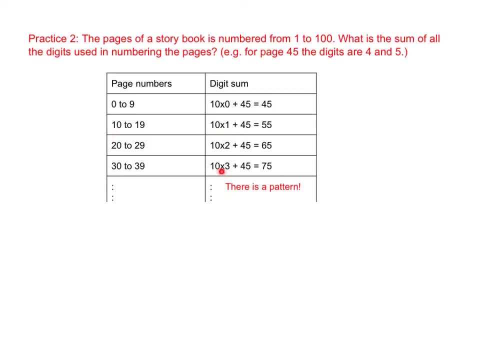 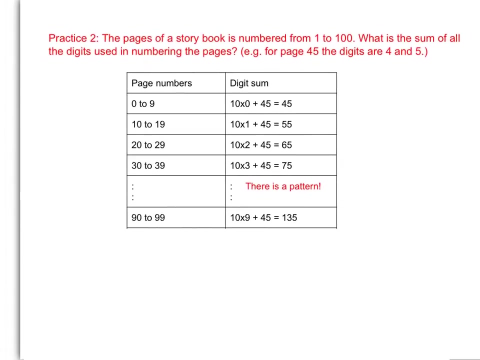 I have 10 times 1. And 10 times 2., 10 times 3. And so on. So if you see this pattern, then we can omit a lot of work and pretty much jump far away down. I'm looking for 1 to 100 page numbers. 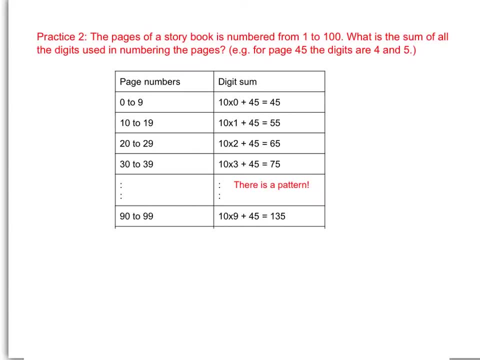 So 1 to 100 right here. So the last group I'm going to list out is 90 to 99.. I use the same pattern here. So I have 10 times 9 plus 45, which is 135.. 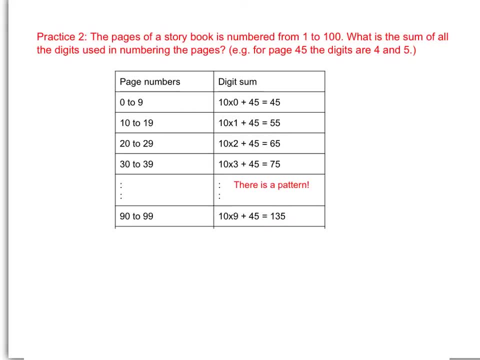 And then, when you get there, the only page that is still missing is the last page, page 100.. 100 is digit 1 and 0 and 0. So I just added these 3 digits together And I get 1.. 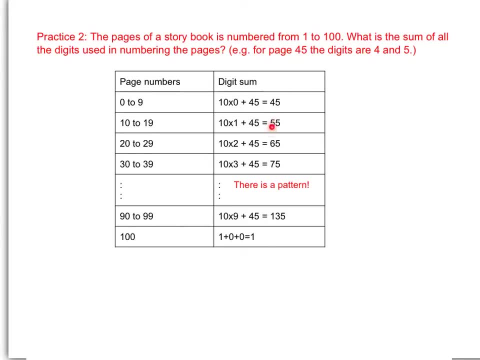 OK, Now what I need to do is just to add up all these sums- 45,, 55,, all the way to 135- and add 1 more to it. That will be the answer to this problem, And I come up with this expression. 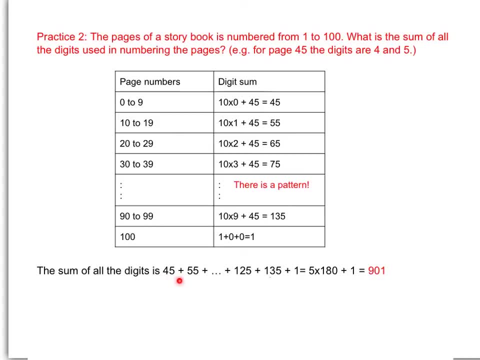 Now. So I need to add 45,, 55, all the way to 135 and add 1.. And Actually I noticed something very interesting, Because 45,, 55,, they increase by 10 for each number, right? 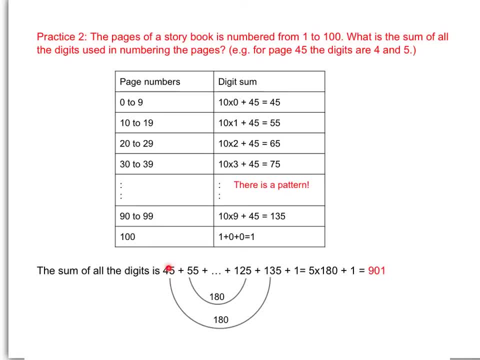 And I noticed that if I group the first one and the last one, I get 180.. I group the second one and second to the last one, I also get 180.. This is actually a very classical way of adding sums like that. 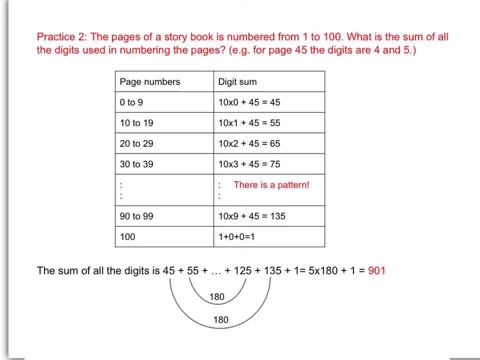 Adding numbers like that, But I will use another lesson to talk about that. So once you notice that. so let's find out how many pairs of sums we have here: 45,, 35, that's 1 pair Actually, from 4 to 13,. 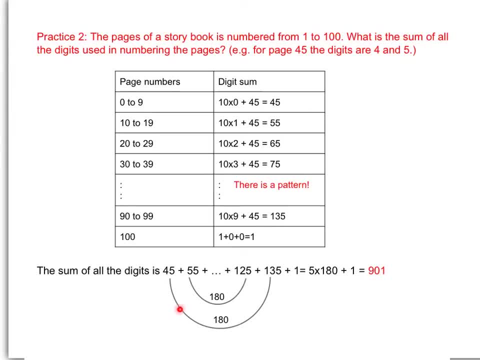 there are 10 numbers. So if I pair up each 2, then I will have 5 pairs. That's why I have 5 times 180.. But don't forget this 1.. So add them all together, I get 901.. 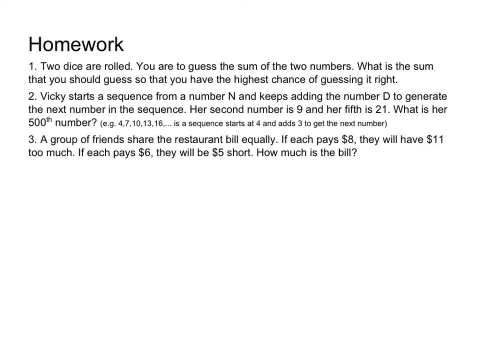 Here is the homework Now. although there are many ways to solve a problem, you are highly encouraged to use what you have learned today, which is making a table to solve the problems- Some problems. there are other ways to solve them if you know a higher level of math. 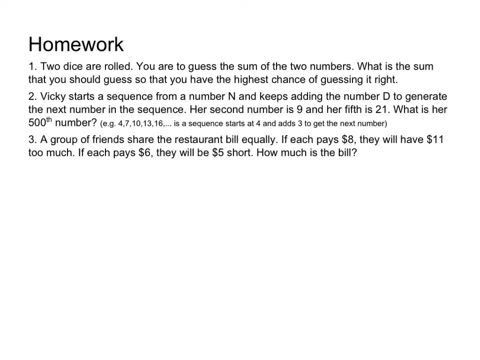 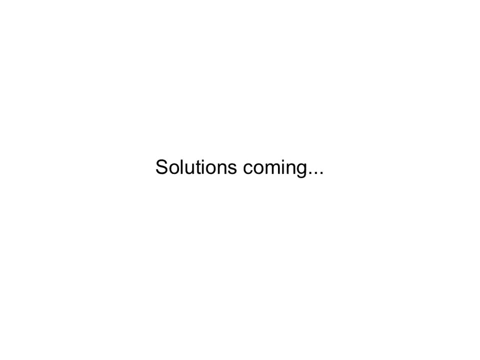 But if not, a table is a good choice for these problems. When you are ready, you can move on to the next page to look for the solution. So now, please pause. Here comes the solutions. Okay, if 2 dice are rolled, 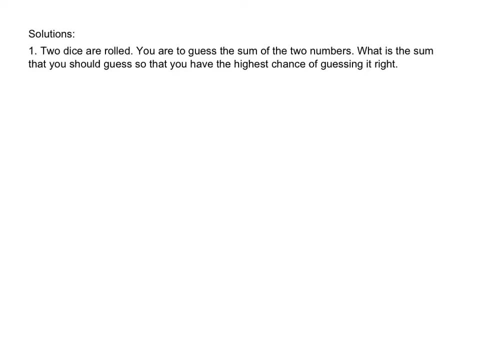 and you are to guess the sum of the 2 numbers shown. what is the sum that you want to guess, so that you have the highest chance of guessing it right? And I use a table to display the possible numbers and their sum. And this table will have. 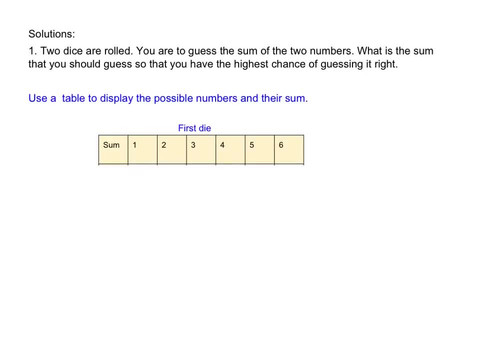 the numbers that can come from the first die and also the numbers that can come from the second die, And I add up the 2 numbers to get the sum, Like if the first die is 1, the second die is 1, then the sum is 2.. 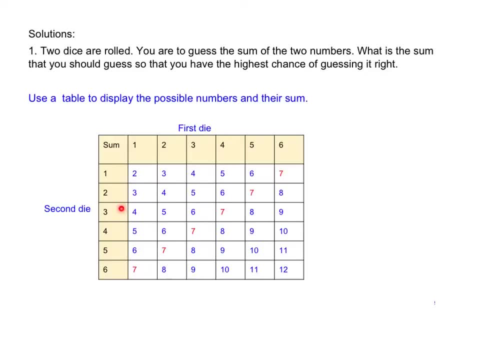 If the first die is 4, the second die is 3,, then the sum is 7.. Now, after I populate this table, I notice some very interesting pattern here. You can pretty much see the numbers go in diagonal, And you should not be too surprised about that. 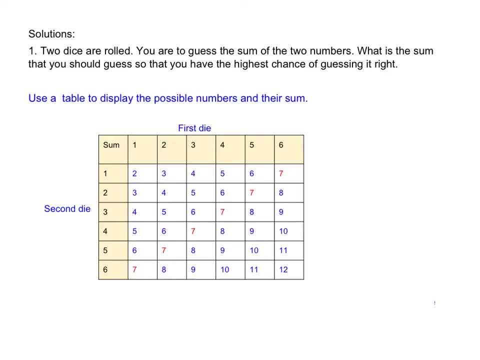 because when we go diagonal, that means one die gains 1 and the other die loses 1.. And that's why the sum stays the same. In this table, we also visualize that 7 occurs the most number of times, And because of that 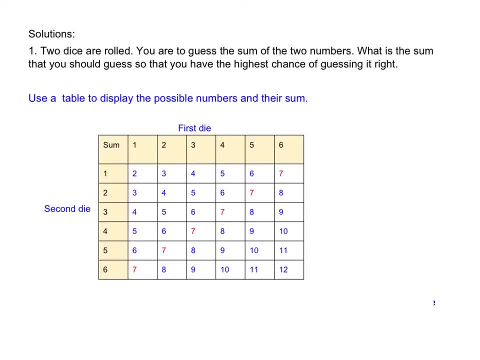 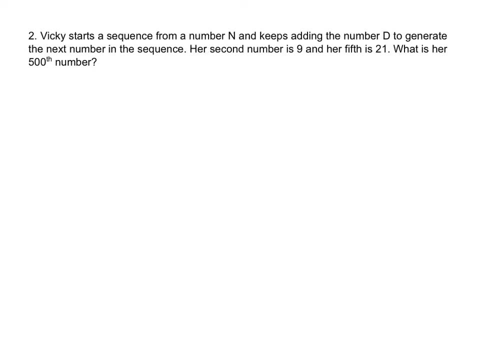 if you guess 7 is the sum of the 2 numbers, you have the highest chance of getting it right. In this second problem we are dealing with a sequence. A sequence is an ordered list of numbers, that each number can differ from the previous one. 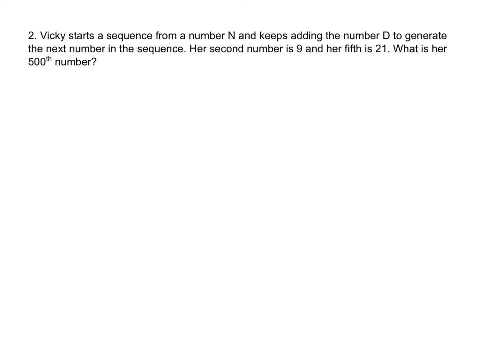 by the same amount. So in this problem, Vicky starts the sequence from number n and keeps adding the same number, d, to generate the next number in the sequence. What we are given is her second number is 9 and her fifth is 21.. 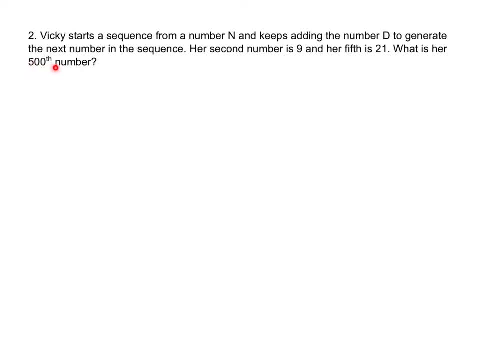 And we are asked to find the 500th number in the sequence. Now, of course, you are not to write the numbers like from the first one all the way to the 500th one, because this will just take forever. We can use a table to help us. 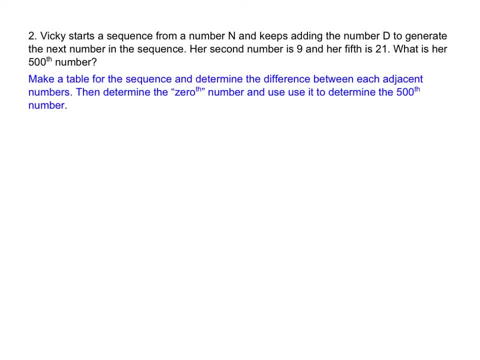 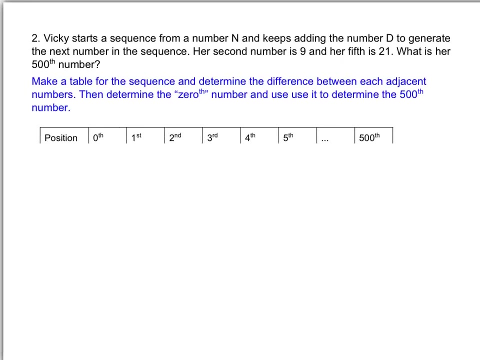 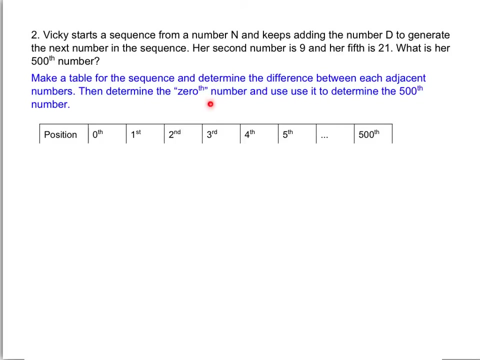 This table will help me find the pattern in the sequence. So in this table I'm going to determine the difference between each adjacent numbers And I also want to determine the 0th number. And the 0th number is quite useful, which I will explain in a second. 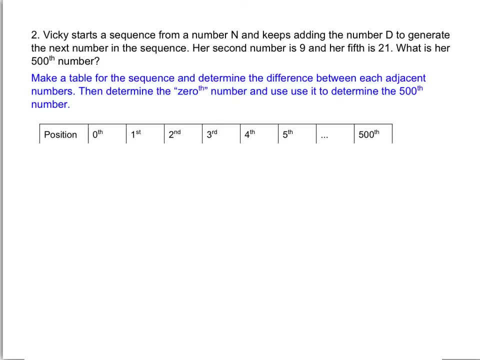 I can use this 0 number to determine the 500th number. So in my table I have the position of the sequence, The 0th position, first position and so on. Now, usually we start the sequence with the first member. 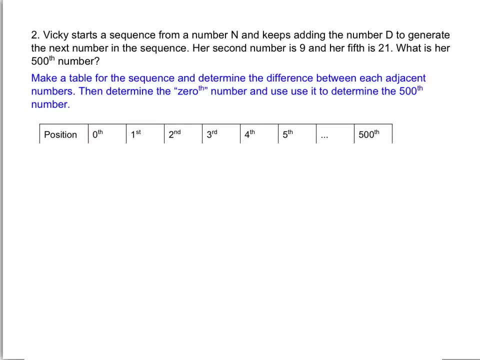 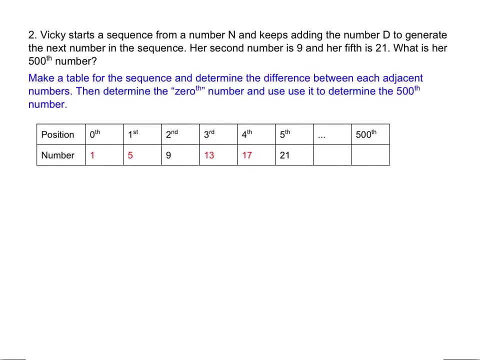 I'll explain why I have this 0th one, because I found out it's quite helpful and handy. Okay, and then in my second row of the table, I list the numbers. What I'm given is the second number. The second number is 9.. 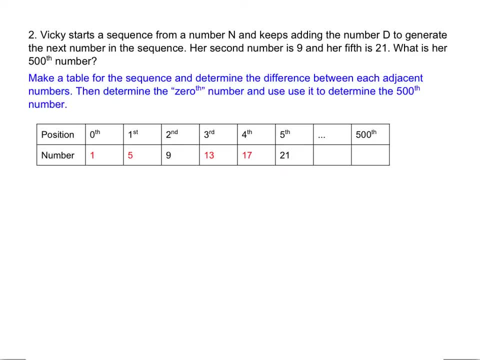 The 5th number is 21.. Now, from these two numbers, I need to determine the difference between each adjacent number From the 2nd to the 5th. I'm having 3 jumps, 1 jump, 2 jumps. 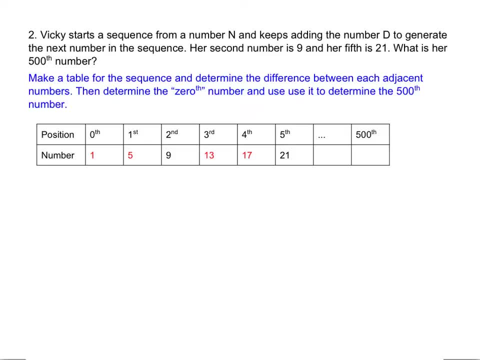 3 jumps In 3 jumps. the difference is the difference between 9 and 21,, which is 12.. So each jump has the difference of 4.. So I figure out these two numbers, But actually what I want to find out more. 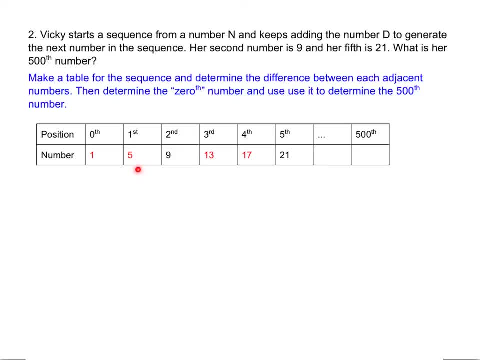 is my first number, So I can go backward by subtracting 4.. And, as I said, I wanted to find my 0th number, which is 1.. Now, why do I want to find this number? Because that can be very useful. 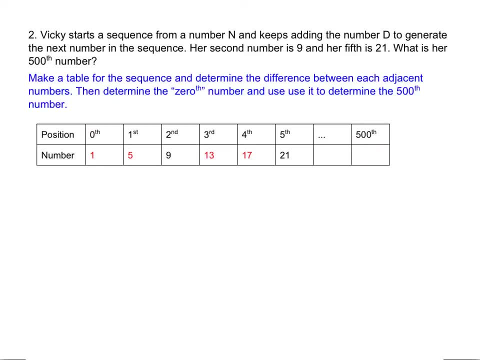 for me to find whichever member in this sequence. So continue to move forward. I found out the difference. d is 4, the starting number n is 5, the 0th number is 1.. Now make some observation here. The first number: 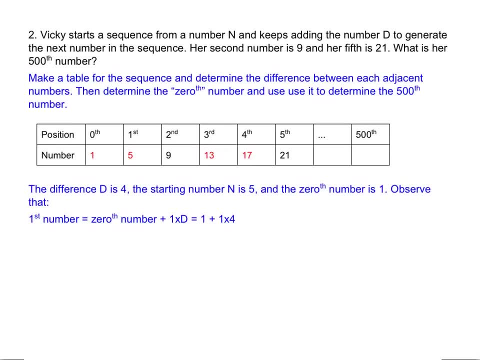 5, is from the 0th number at 4.. Right, The first number is the 0th number plus 1 difference, So it's 1,. this is the 0th number and 1 difference, which is 4.. 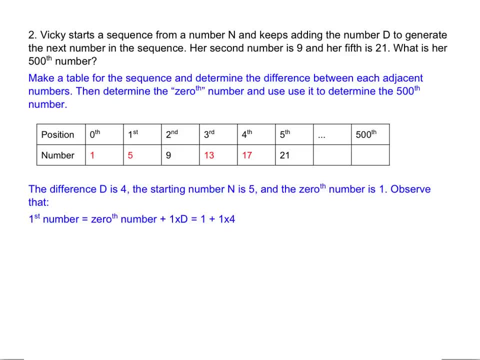 So it's that which is 5.. And I also observed that the second number is the 0th number at 4, at another 4.. So it's 1 plus 2 difference 2 times 4.. And I continue to list a few more. 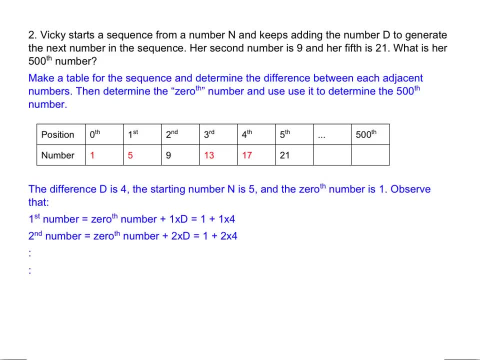 And then I see this pattern. So if I want to do the 500th number, I use the same pattern. I start with the 0th number. That's why I want to start with this one. I'm looking for the 500th one. 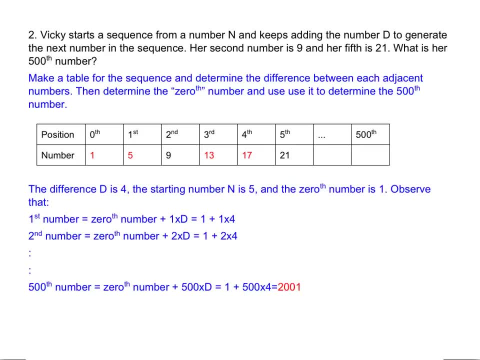 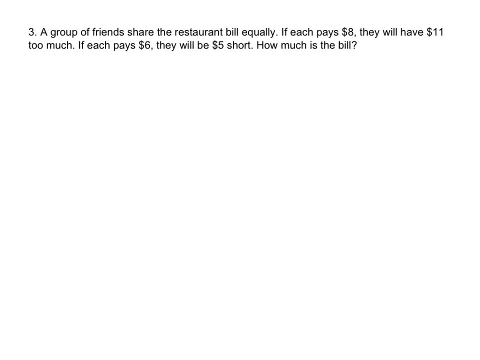 So I will just add 500 difference. So it's 1 plus 500 times 4.. The answer is 2001.. Here is the solution to the last problem. Again, there could be more than one way to solve it. If this way is different from yours, 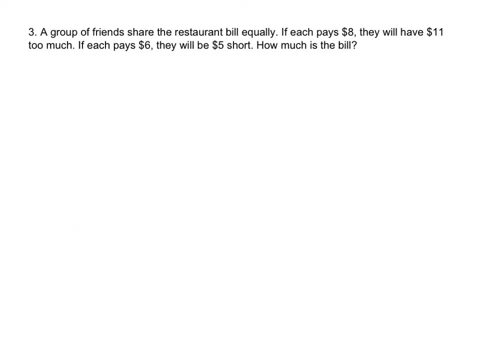 yours may be fine too. I use a table to test different number of people and the bill amount, So since we don't know how many people are in the group, I listed a couple of possible ways So I could have 1 person in the group. 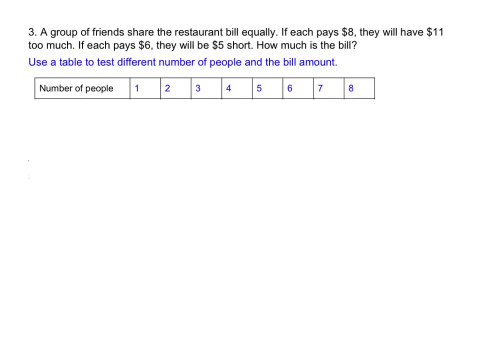 or 2 people And all the way to 8. And then for each possible number of people in the group, I also examine the bill amount And this is what I got for the table. So what is the bill if each person pays? 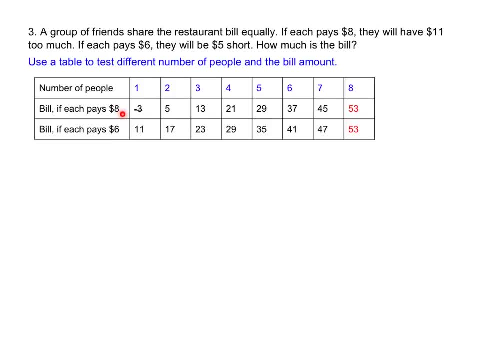 $8?. If there is only 1 person and the bill would be quite interesting, because that person pays $8 and then we have $11 too much, That means the bill must be a negative number. That's why I cross it off. 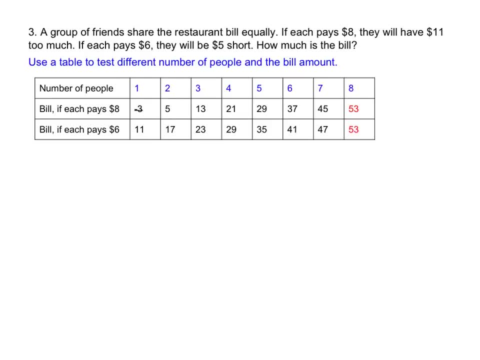 And if we have 2 people, then it started to make sense a little bit. 2 people each pays $8.. And so they would have paid $16 in total, But then I have $11.. They have $11 extra. That means the bill must be $5. 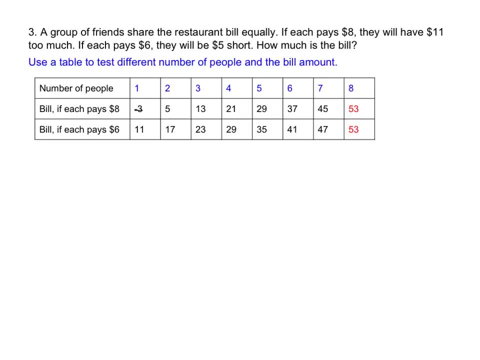 And using 2 people again. if they each pay only $6, that means we only collected $12.. And it says they would be $5 short. That means the bill must be $17.. Now these 2 dollar amounts don't match. 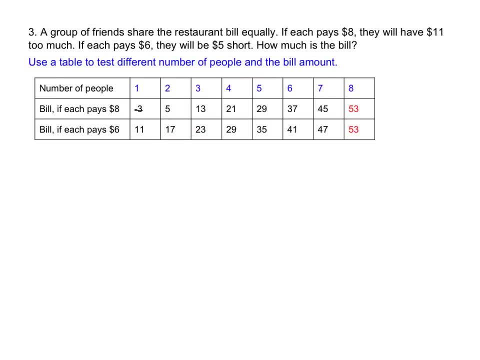 One says the bill amount is $5.. The other says the bill is $17.. They don't match. So we try another one, Try for 3 people Using the same way, to test it out And eventually we will get to the right answer. 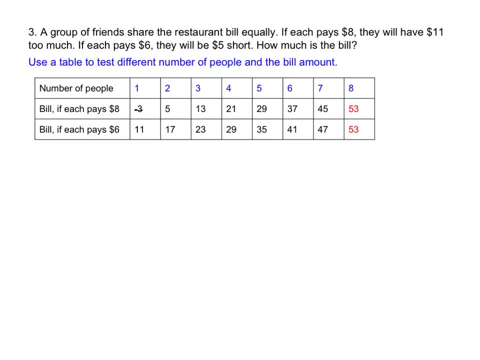 But do we have to try that many times? We can make some observations here. So the difference between these 2 bills is $12- $10 and $8- $6. Do you see the trend? So maybe knowing that we want those 2 bills to be the same, 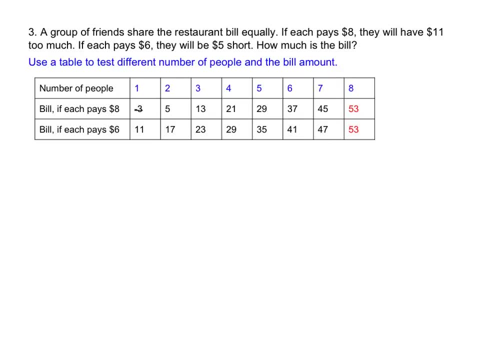 so perhaps we can jump a couple of them. If we see that each time the bill difference is narrowed down by $2, we can perhaps use that information to jump to the answer pretty fast. Well, I hope you learned something interesting today and can help you to solve some problems down the road. 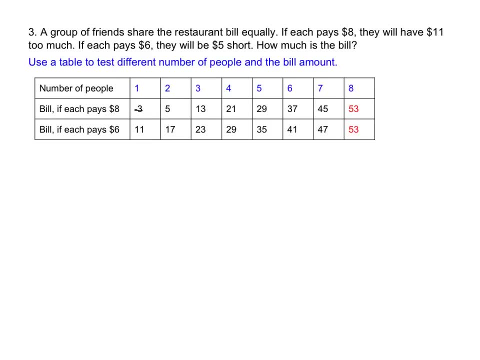 Please do not forget to watch my other videos in problem solving. Goodbye.